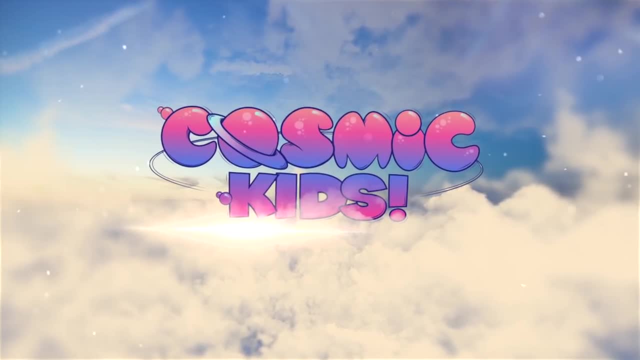 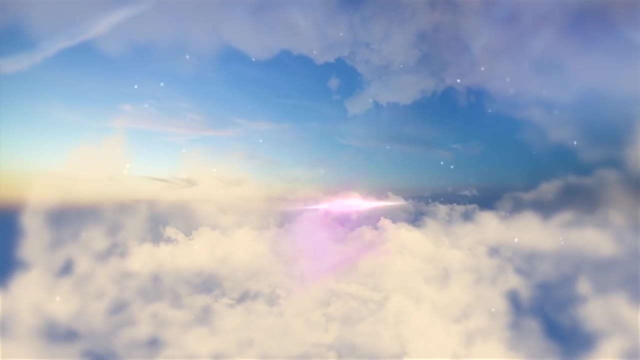 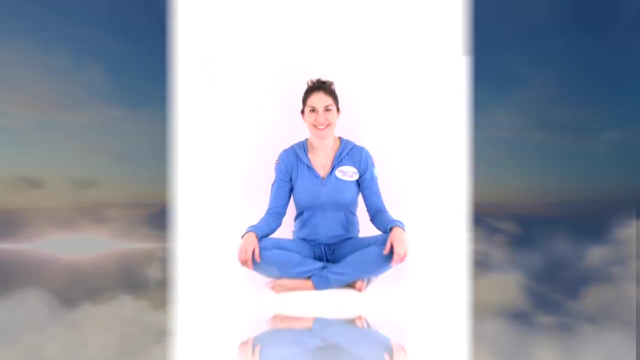 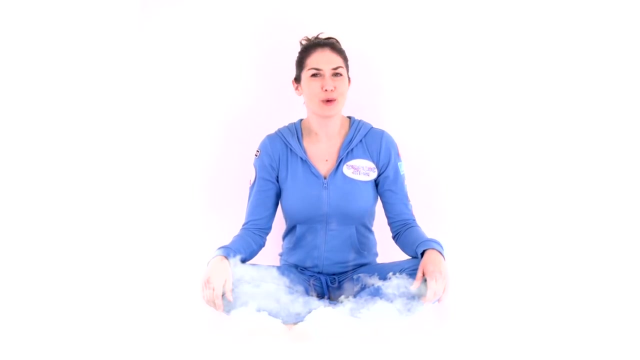 Hello everyone. welcome to the Cosmic Kids Zen Den. This is your place to feel all calm and relaxed and to help us get healthy and happy in our minds. First, let's get comfy, sitting on our bottoms with our legs crossed or, if you like, you can lie down. We take. 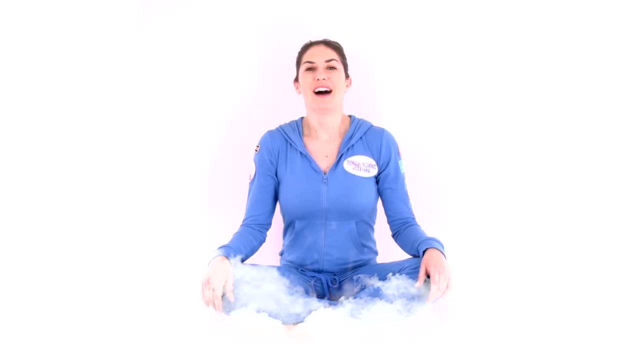 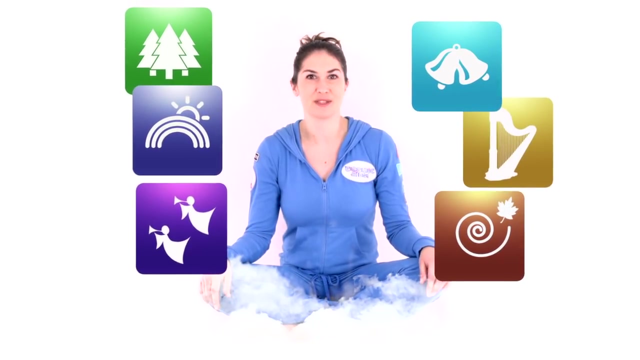 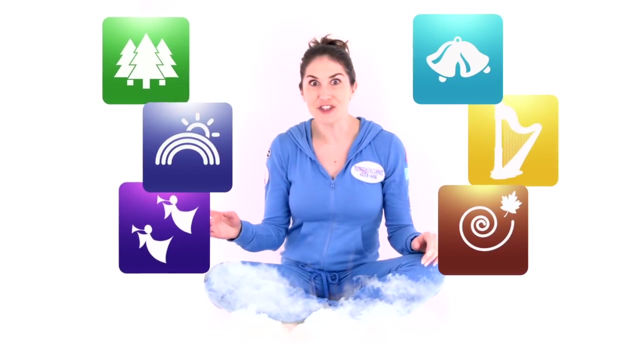 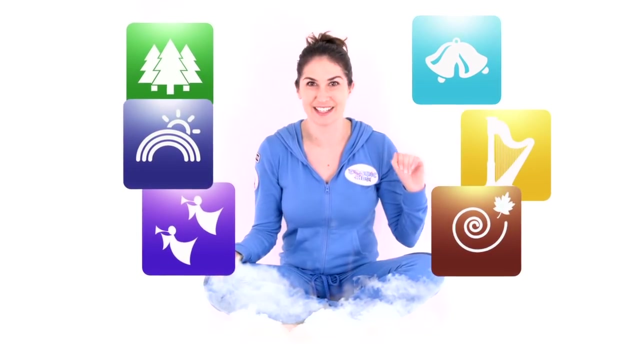 a big deep breath. Ah, that's better. Now let's get the Zen Den ready so we can really enjoy it. We need music. Here are some sounds to choose from. Let's pick the ones that help us feel. just right: The sound of a harp, Angels singing And some twinkly bells- Perfect. 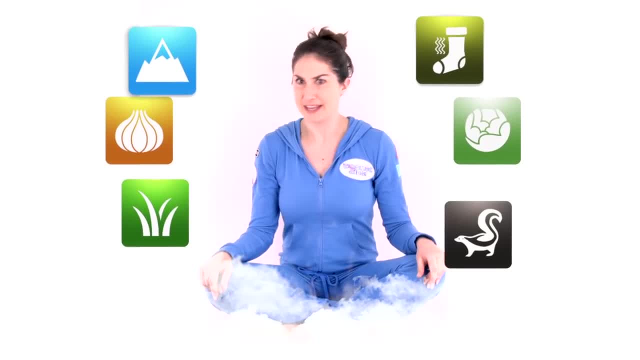 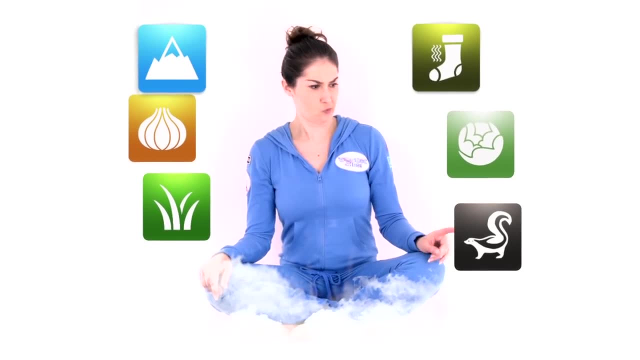 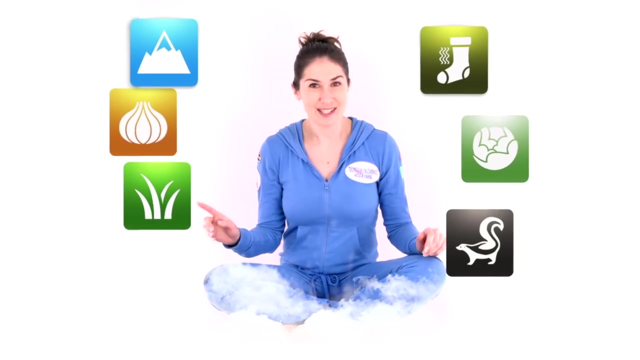 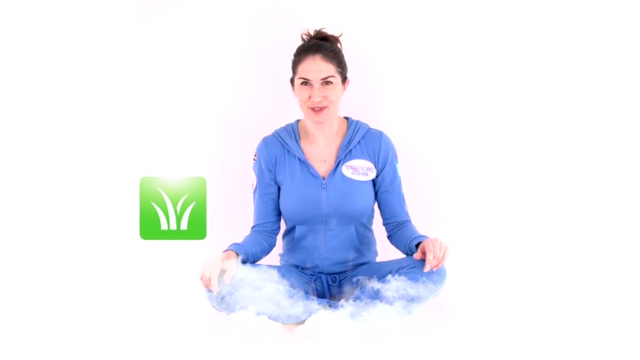 Now for the smell. Oh, look at these. What have we got here? We've got a little bit of these here: The smell of cabbage, The smell of hay. You know skunk smell. No thanks, Here's one. Let's smell the freshly cut grass. Ah yes, such a wonderful smell from springtime. 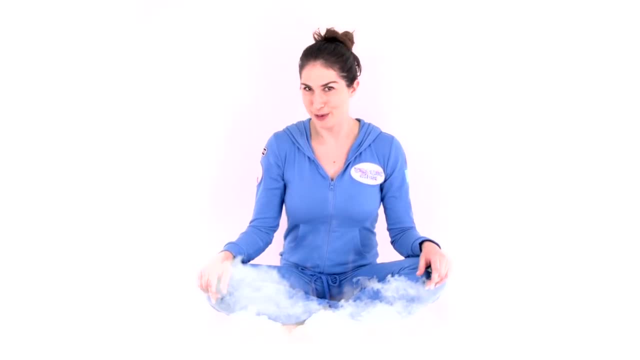 There's a little word we sometimes use when we think something belongs to us: Mine, mine, mine, mine. I wonder if you can think of a time when you have said it maybe in one of those ways, every time we say it, we probably have a really strong feeling. at the same time, we might feel angry or frustrated, or sad or frightened that we've lost it and we're never going to get it back again. the thing we think is mine might not even belong to us, but we still say it. I wonder: have you ever been? 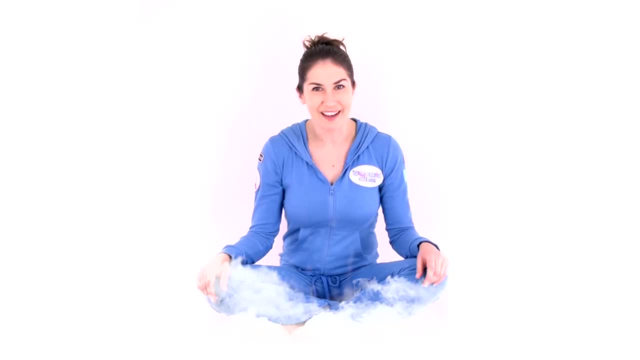 to a playground where you play on the slide, the roundabout and the swings. maybe there's one nearby to where you live, where you go and play. let's go on a journey to a playground now. listen to the words and make the pictures in your mind. you might find it. 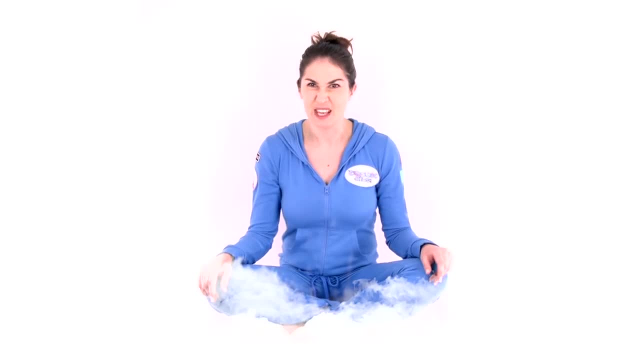 easier to close your eyes or, if you prefer, keep them open. you love going to the playground. it's a place you really enjoy as you get to go on all the fun things like the playhouse, the slide, the seesaw, the merry-go-round and the swings. 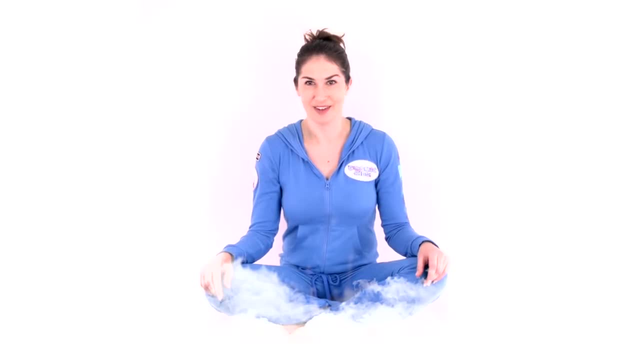 there's a special swing that you always go on. you love being pushed on that swing, swooshing up and down, higher and higher. you can't wait to get there today to have a go on it. you walk to the playground with someone from home, maybe mommy or daddy, or a grandparent or 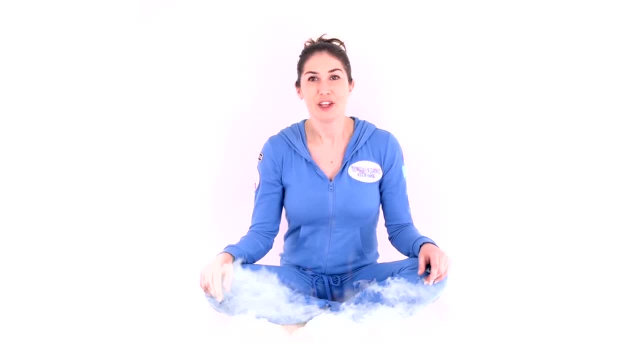 someone who looks after you. you hold their hand as you walk. as you get nearer, your excitement- 느낌이還有 your excitement grows for what you now think of as your swing, My swing, Mine. As you arrive at the playground, you see it's quite busy with lots of children playing on the 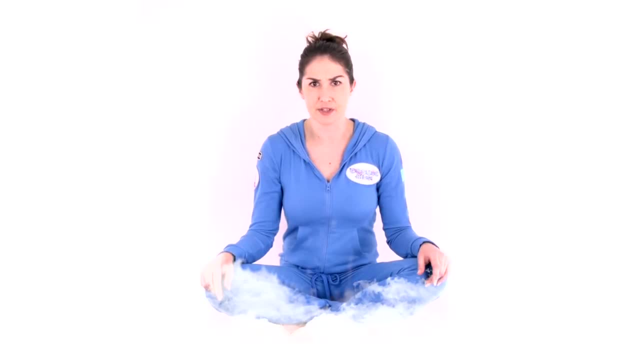 slide the merry-go-round, the playhouse and the swings. Your eyes fall on the swing you think of as your swing and there is a little boy on it being pushed by his grandma. He's laughing and she's enjoying making the swing go higher with. 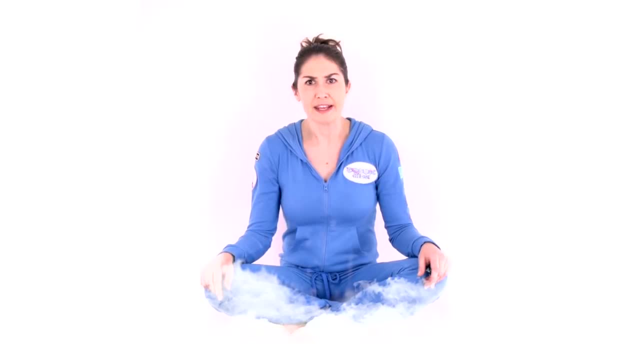 each push You think, hey, that's my swing, he needs to get off, it's mine. Maybe you say it out loud to the person you're with. A feeling comes up inside you. What is that feeling? Stress, Anger, Fear, A big 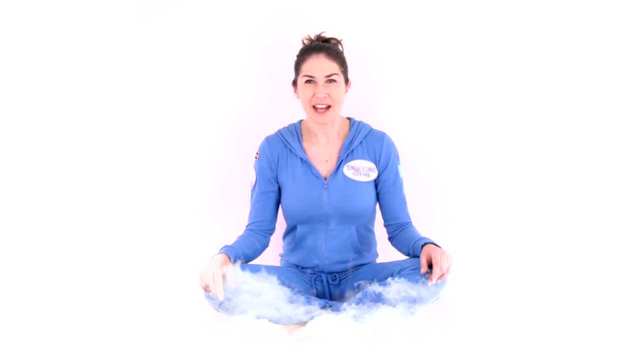 change, Jumble of all of them. Can you notice the feelings? How do they feel to you? Now ask yourself what makes this swing mine. Does it really belong to me? Hmm, no, it doesn't really, but you might still have that mine feeling. What might be the best?